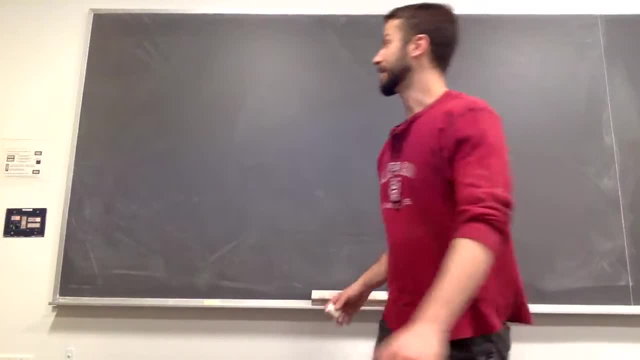 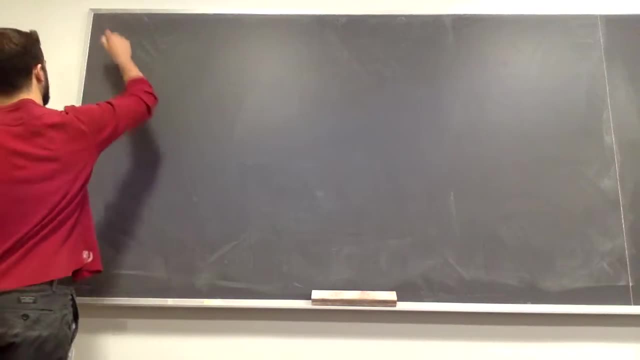 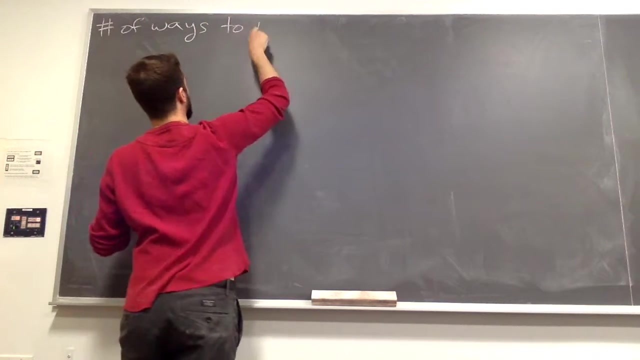 Okay, so we're going to do a counting problem. Okay, we're going to think of a pretty pretty, pretty quick, pretty like succinct prompt for this problem. We're going to try to count the number of ways to pair 2n people. 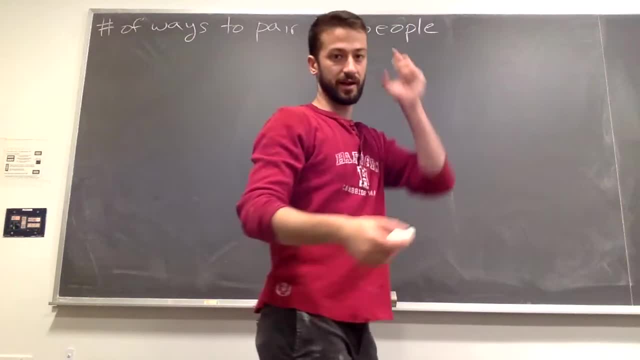 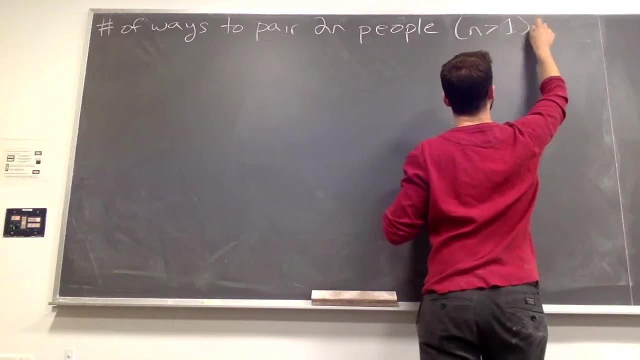 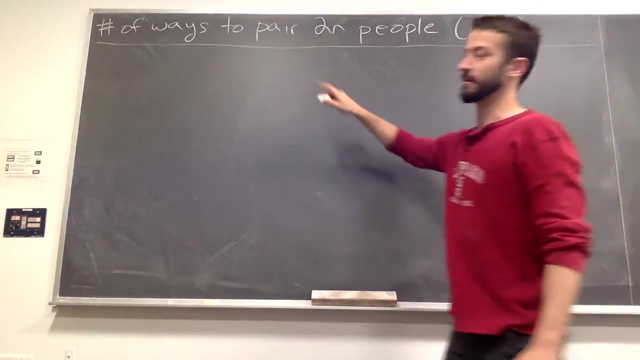 I'm going to say, just so this isn't like a trivial problem. we're going to say n is a positive integer that's greater than 1.. Okay, that's it. That's our problem. The proper way is to pair 2n people such that n is greater than 1.. What does this? I mean, we kind of know, we know what pair means, but what does pair mean in this context? What does it mean to pair the people? 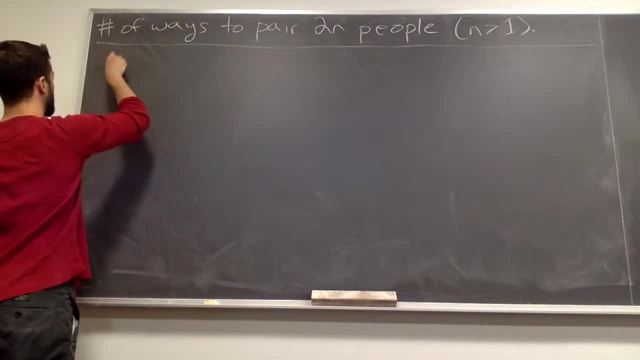 Let's consider a simple case. So we're going to consider a case when n equals 2.. Okay, so n equals 2, that means we have 2 times 2, we have 4 people. Let's just label the people a, b, c and d. Nice and easy games, Okay. 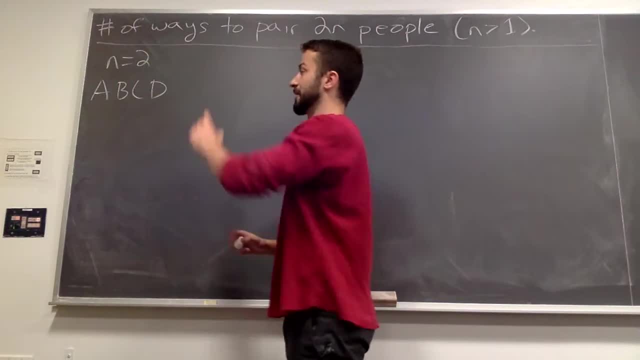 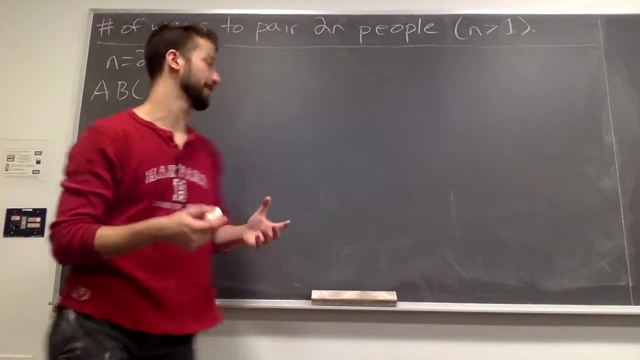 So in this case, with 4 people, it's actually very easy to count the number of ways to pair them, One permutation or one like yeah, one specific permutation of this pairing is to put all these people into pairs, so to pair them off. 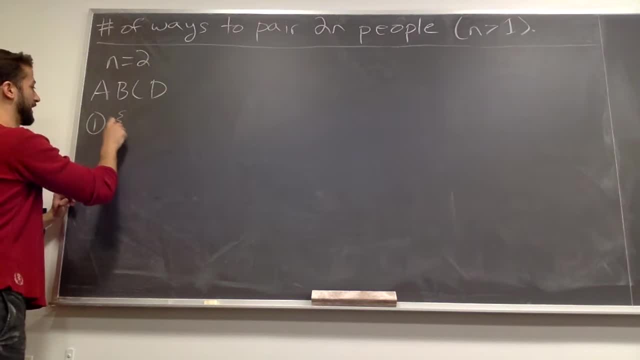 And you'll see what I mean when I actually do it. So the first permutation is pairing a and b and pairing c and d, So we put everyone into pairs. We have two pairs, but this counts as a single permutation. This is one way to pair everyone. 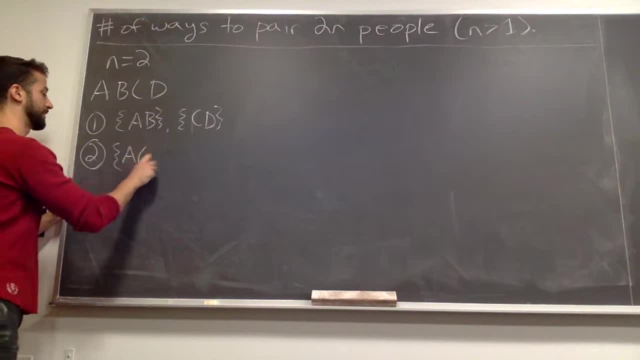 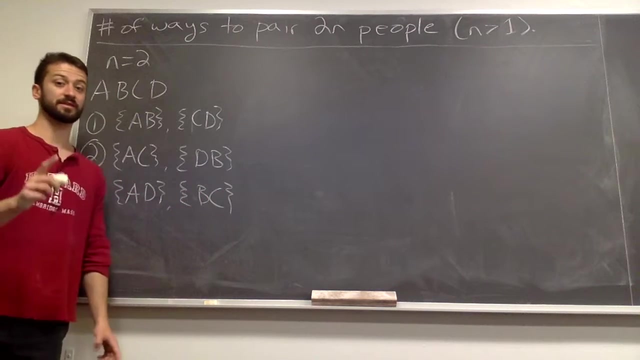 A different way is to say a and c, pair a and c and then pair d and b. And the third and final way is to pair a and d and then pair b and c. Okay, A quick thing to note. it doesn't matter. it didn't matter if I would say c and d and then a and b, right? 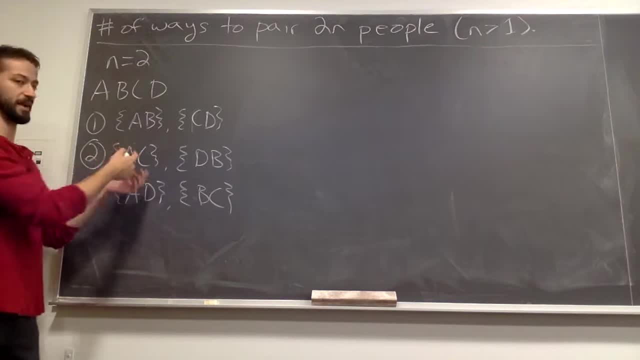 It doesn't matter if I flip flop the pairs. It's still wonderful. It's still one permutation. we still have a pair of a and b and a pair of c and d, so that that order doesn't matter. And also the order within pairs doesn't matter. It wouldn't matter if I wrote b and a instead of a and b. 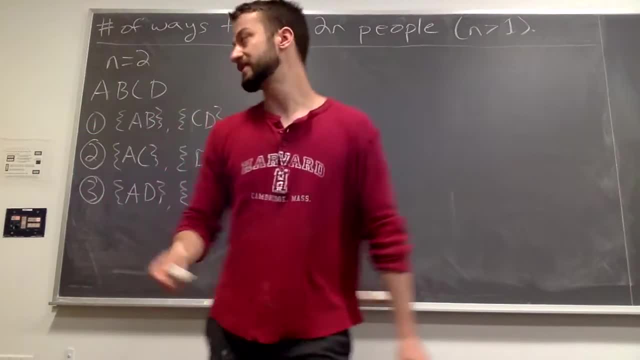 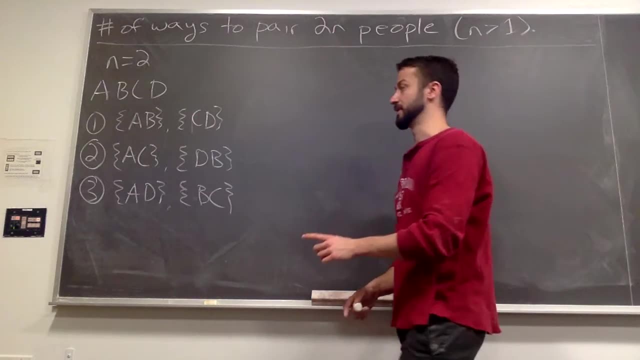 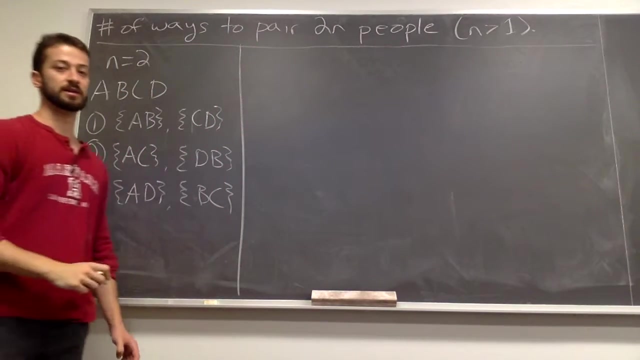 It's still a pair of a and b. So this is saying that we have three total permutations in the case where n equals 2.. We want to solve this for a general case of n. Okay, So this looks pretty. looks a little intimidating the first time you see it. I think for sure. 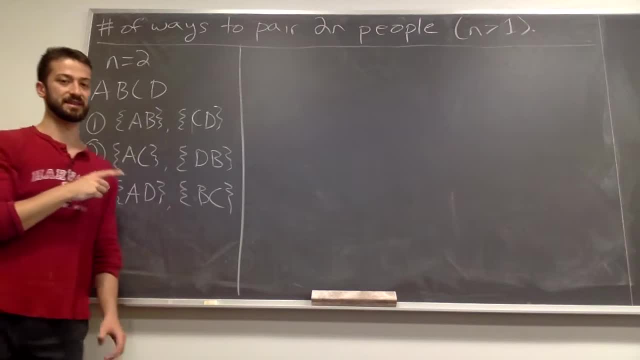 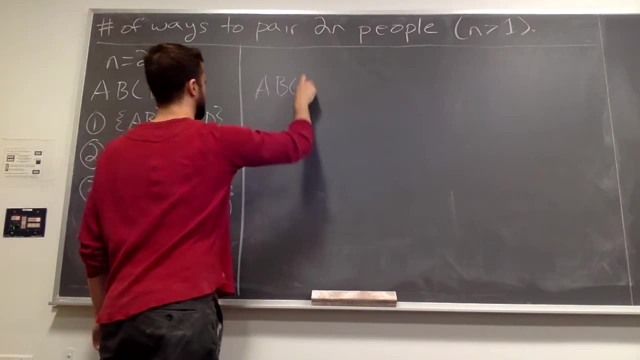 The way I want to think about it is extending this kind of like a b, c, d thing right And say calling people letters. So let's think of: we have a b c d, dot, dot, dot dot, right. 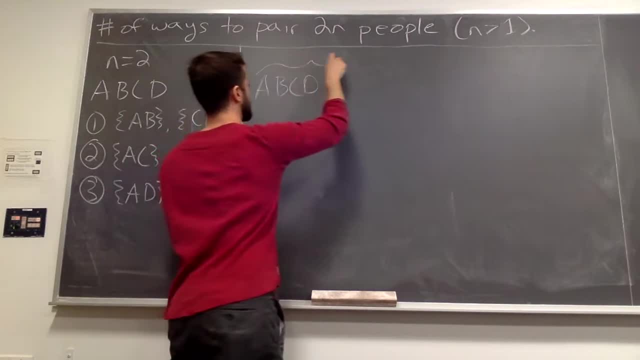 And this goes on. this goes to 2n people, 2n letters. Okay, And the way we're going to think about generating pairings, make sure the dot, dot dot is clear. The way we're going to think about generating pairings is we're going to randomly permute this word, right? 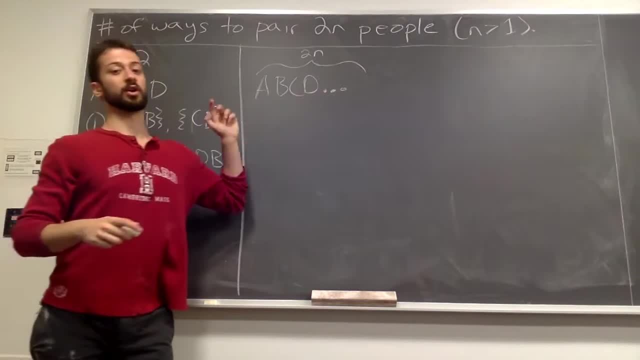 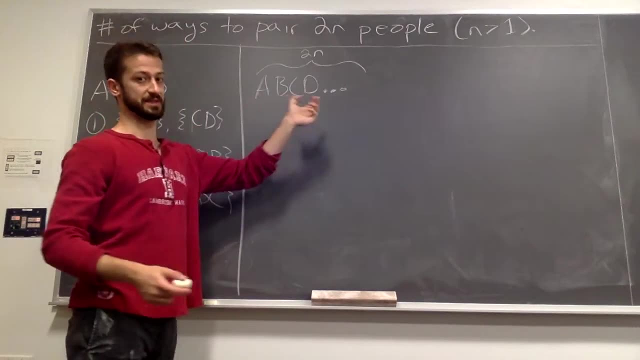 Quote: unquote word: Randomly permute this word We're going to go through and two at a time we're going to pair the people. So let's say I draw a random permutation. Let's say this is my random permutation: a, b, c, d, et cetera. 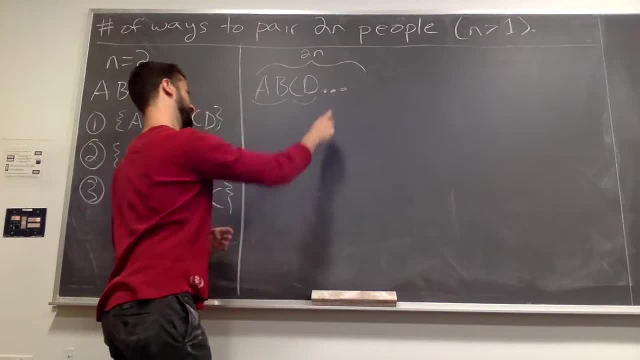 I'm going to say: okay, an, a and b are a pair, c and d are a pair, The next two people are a pair, the next two people are a pair, et cetera, And that's the way that I'm going to create my pairings. 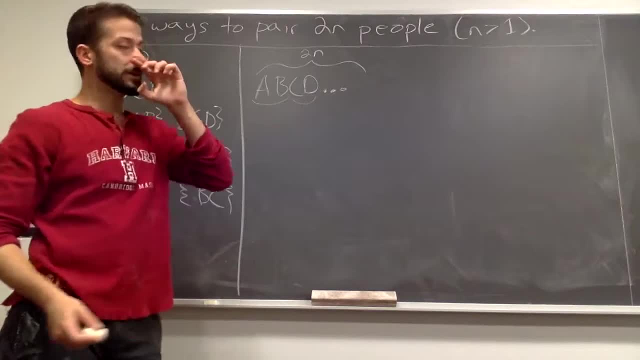 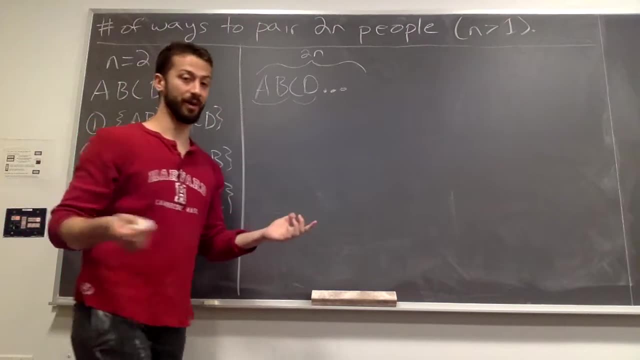 That's one permutation, Okay. So now it's a little bit easier to think about counting the number of ways to do that right, The number of ways to pair, based on this setup, Right away. right, There's two. There's two n factorial ways to spell this letter, to draw this up. 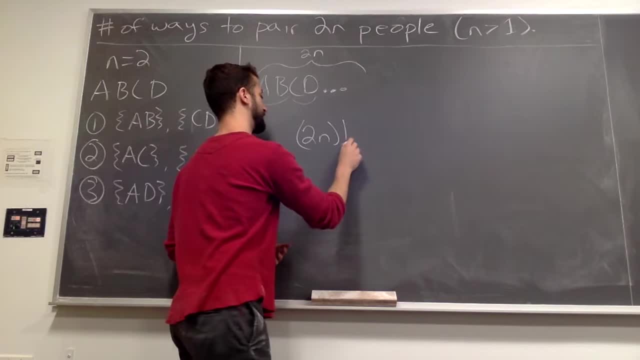 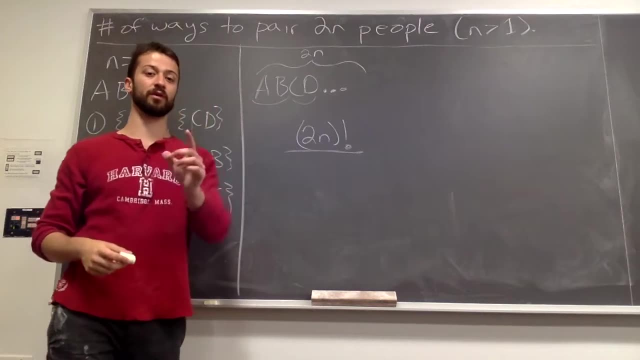 People are unique. There's that number of ways to spell this letter, But spelling the letter is slightly different from pairing the people off right. So that many ways to spell the letter, but we're still overcounting by some factor. How are we overcounting? 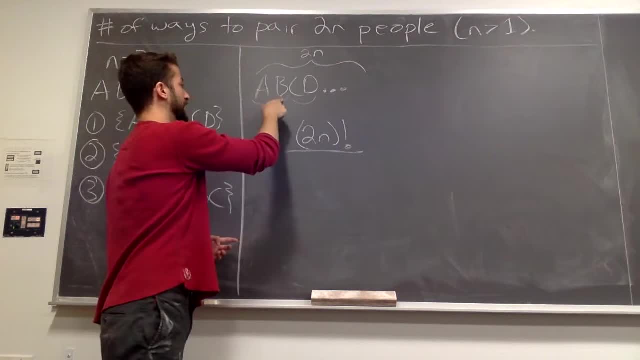 Well, let's think about a and b, right. Let's think about: I have a and b here. What if I had b and a instead of a and b? That would be the same thing, right. Like before we said, order within the pair doesn't matter. 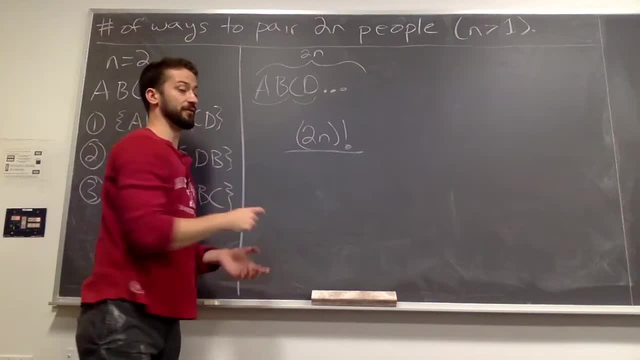 It's still a pair of a and b, So this order doesn't matter. I have two potential orderings, either a and b or b and a, So I have two for that pair And I know I have n pairs right. 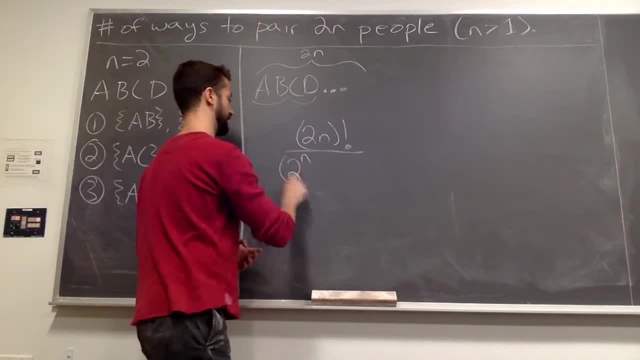 So I have two n people n pairs. So by multiplication we'll have to divide that by two b, So two for this pair, two ordering for this pair, two for this pair, et cetera, et cetera. 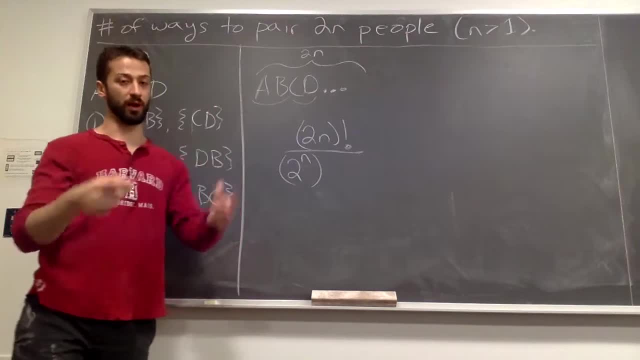 That takes care of ordering within pairs. It doesn't take care of ordering across pairs. What does that mean? Well, it doesn't matter if I have a and b and then c and d, or c and d and then a and b, right? 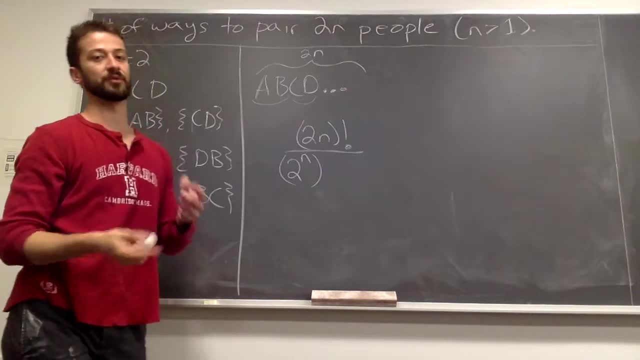 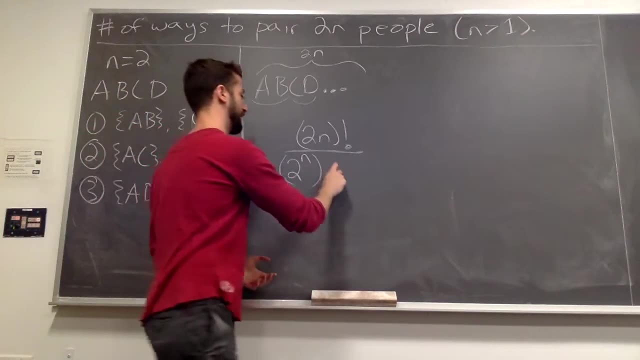 It doesn't matter if this pair. you know, if we swap the pairs around, So we're also overcounting by that factor. So we have n total pairs right Two n people n pairs. We have n factorial ways to line up the pairs. 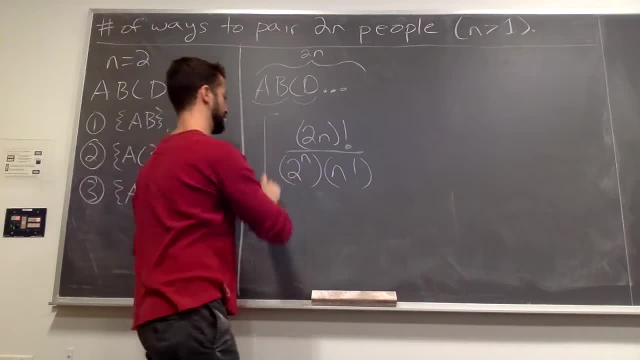 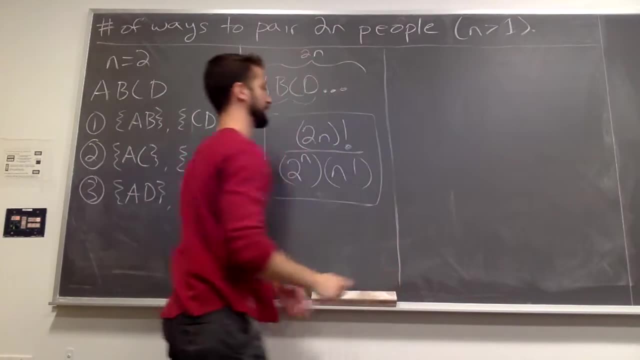 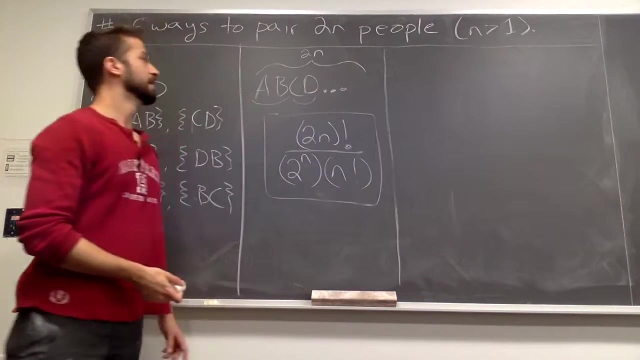 So we divide by that And that's our answer. Simple answer: Okay, An alternative solution that gets you the same result. It's always good to think of alternative solutions because some people sort of just understand different solutions better. You can think of choosing the pairs one by one. 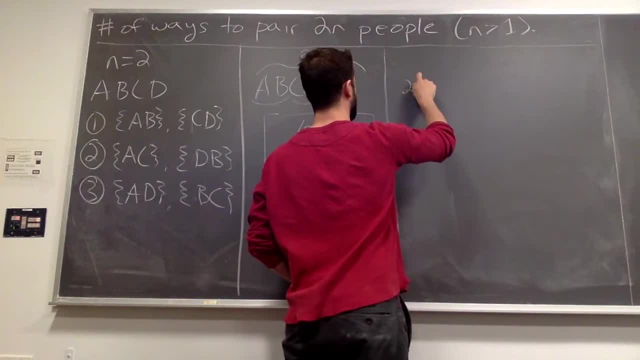 What do I mean by that? Well, okay, so you have two n people. You want to choose your first pair. So you have two n choose two choices for your first pair. You chose that pair. Now you want to choose the second pair. 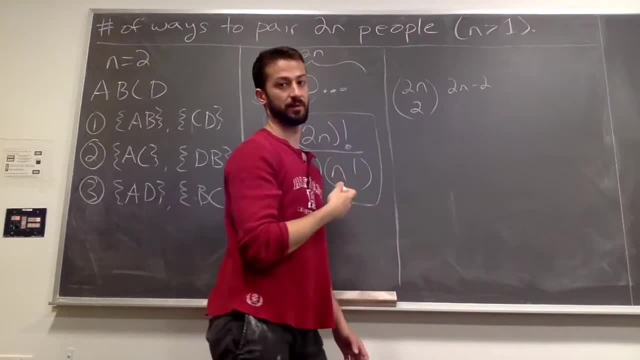 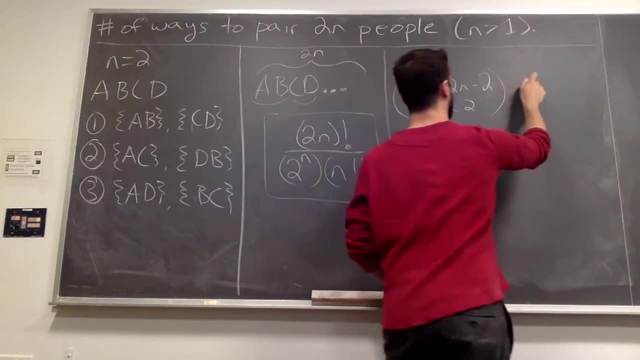 You have two n minus two people left because you took two people out for a pair. Two n minus two choose two. And you keep going until you have the last pair of two choose two, which is just one. Two choose two is one. 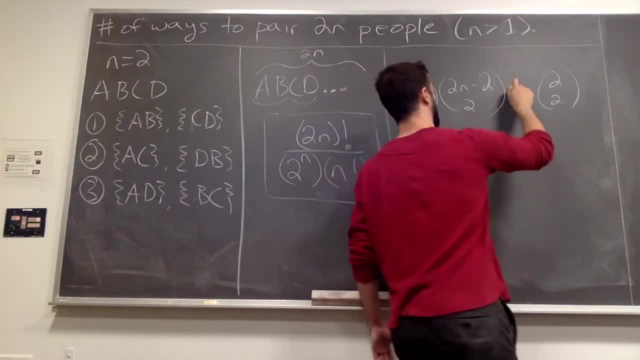 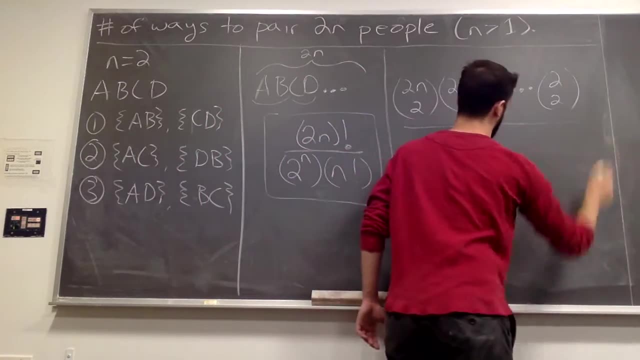 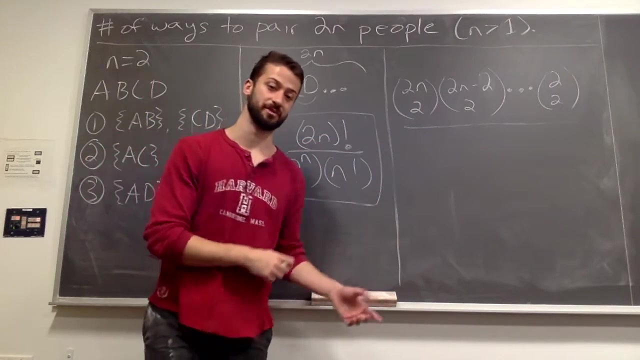 I'm just writing it so you can show the end of the sequence, But you know that's once we get down to the last two people. The one thing we're forgetting is we have to divide by overcountings. Again, this deals, this adjusts for overcounting within the pairs themselves, but it doesn't adjust for overcounting across the pairs. 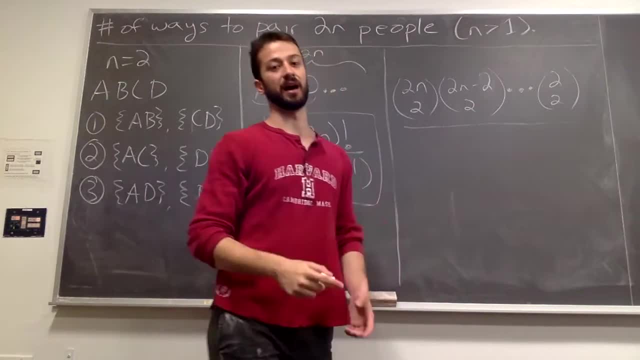 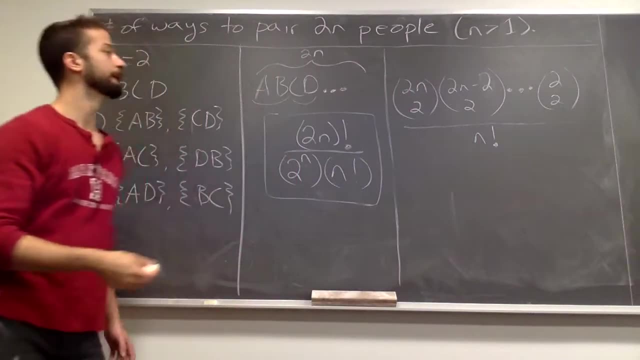 So again, it doesn't matter which pair comes first and which pair comes second. There's still n pairs. You know we want to divide by n- factorial, the number of ways that we can order those pairs. Okay, Does this equal? does our solution here equal this solution? 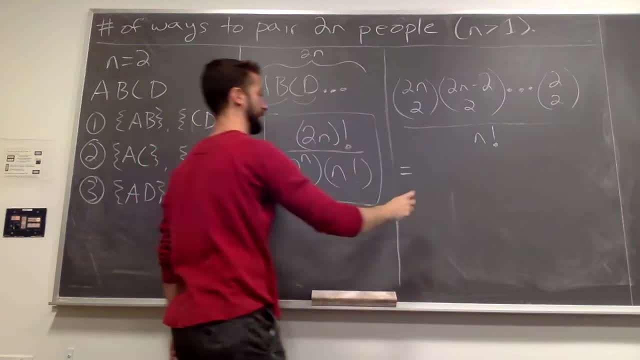 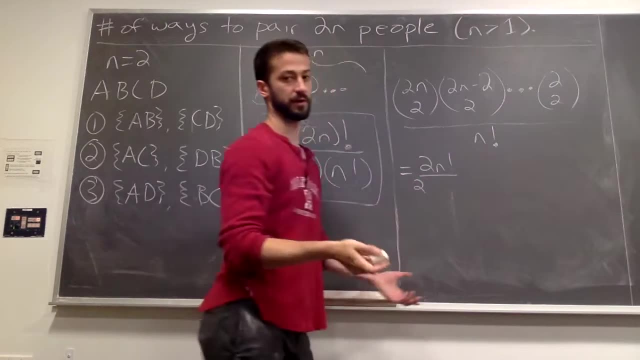 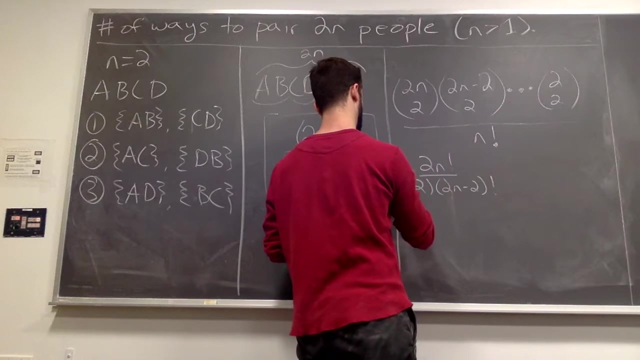 Well, let's check right. Let's plug in the definition of binomial coefficients. So I have two n factorial over two factorial. Two factorial is just two. So over two times two n minus two factorial, That's one term.